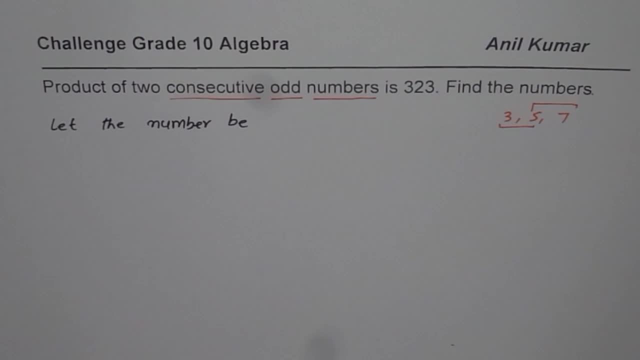 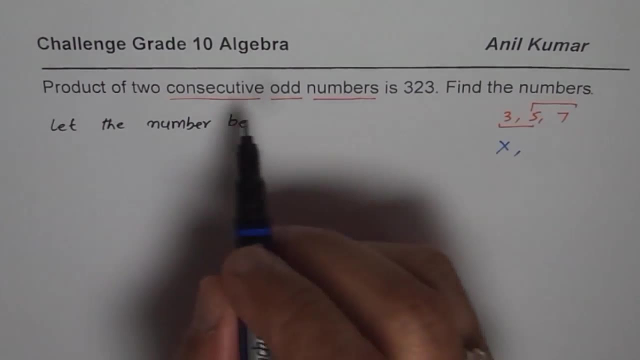 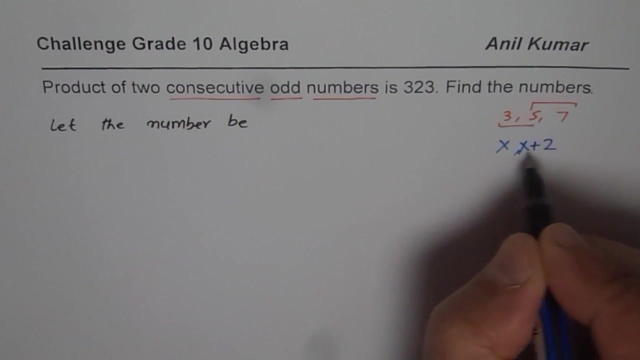 So let us explore a bit so that you can appreciate why I selected what I selected. So if I select one number as x, then the other number should be how much. We are saying consecutive odd. So I should write here as x plus 2, correct? That is how I can get consecutive odd numbers. If 1 is 3, then 3 plus 2 is 5.. I think you got the idea. 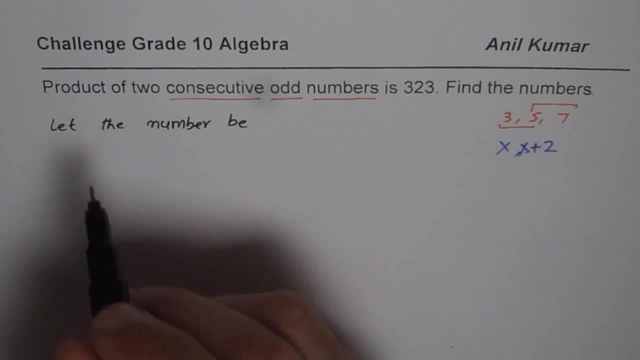 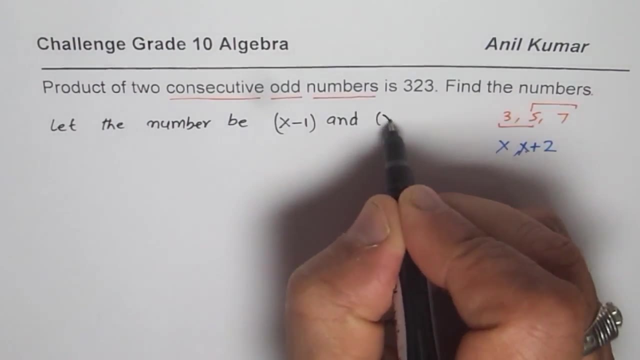 But now, what I will do here is I will say: let the numbers be. how about this? x minus 1 and x plus 1.. Now, if I take x as a number, for example, if I take x as a number, then I will get x minus 1 and x plus 1.. 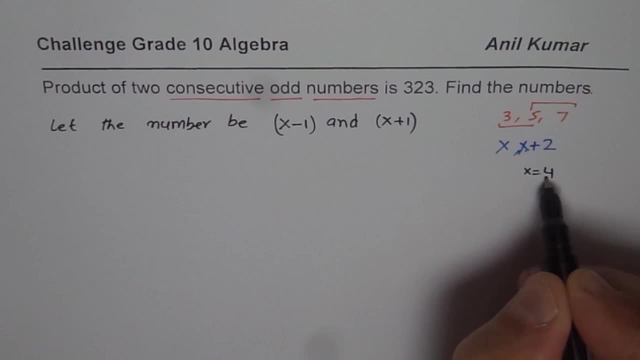 Now if I take x as a number, for example, if I take x as a number, for example, if I take x as a number, then I will get x minus 1 and x plus 1.. Now, if I take x as a number, for example, if I take x as a number, for example, if I take x as equals to 4, in that case 4 minus 1 are 3, and 4 plus 1 is 5, I do get 2 consecutive odd numbers. Do you get the idea? 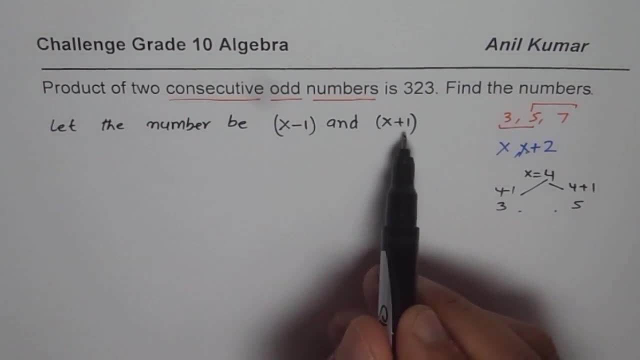 Now, defining variable like this is tricky, smart and helpful. You could go with x plus x 2 also, But I will show you, since you've learned factoring, how that helps to solve this question. and there is one reason why. 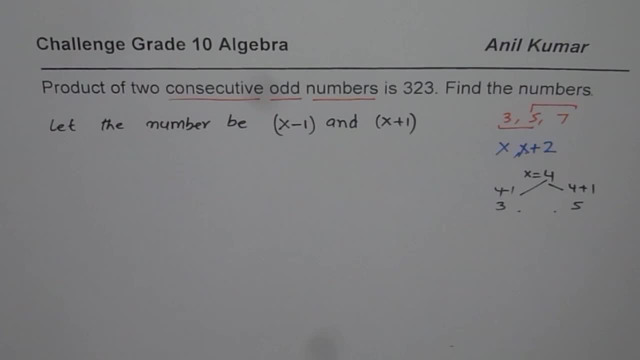 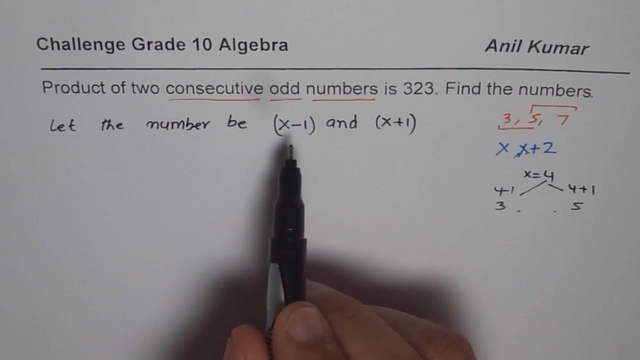 taken this question now once again before you, right? I do have similar question in the list of my videos, right? I'll give you a link for that, okay, so what I say here is that let the numbers be x minus 1 and x plus 1, so they are two numbers which skip. one is included, so they are either odd or 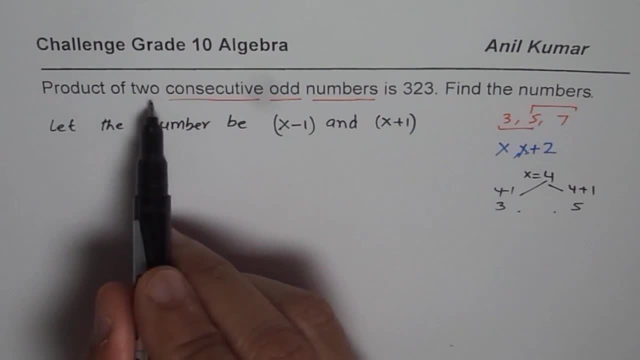 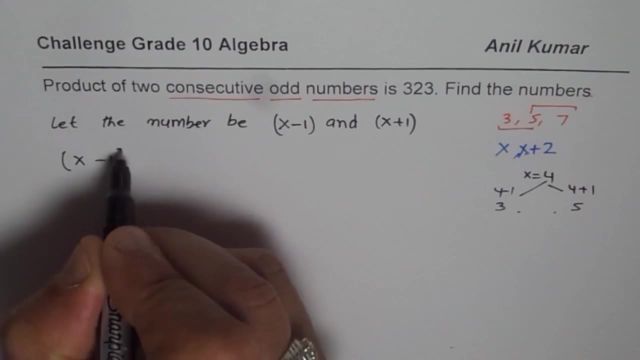 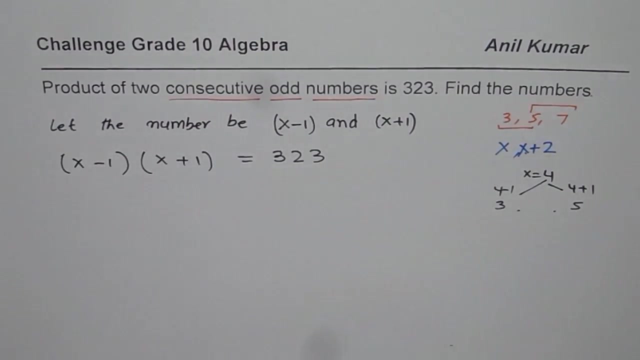 even. but now my equation will be: product of two consecutive odd numbers is 323. so when I multiply them, that means if I do x minus 1 times x plus 1, I should get 323. that is the equation. is translates to equal to right. so product of these two is 323. that is how you form an equation. 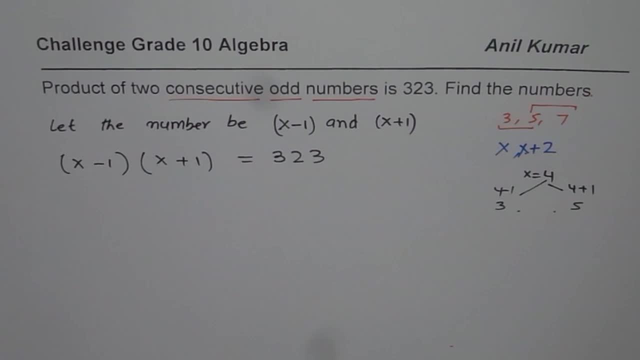 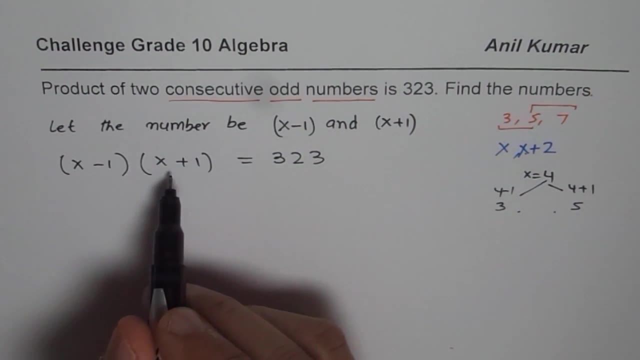 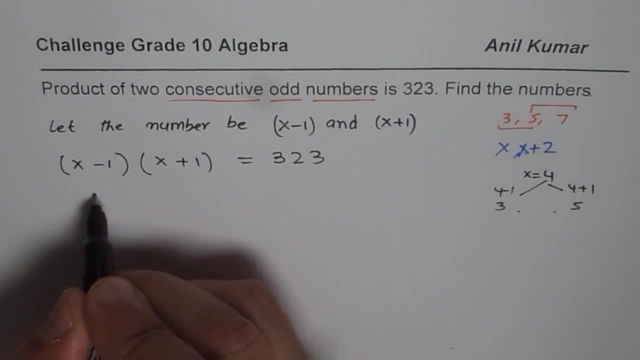 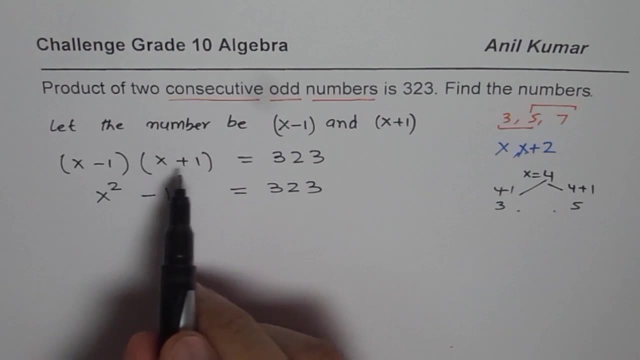 you multiply sum and difference. what do you get? you will get x square minus 1. perfect equals to 323. some of you who have not done this kind of factoring or multiplication of polynomials can apply the distributive property right, and then they will also get the same equation: x- square. 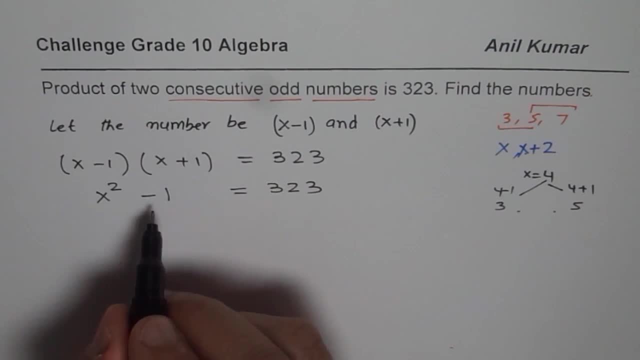 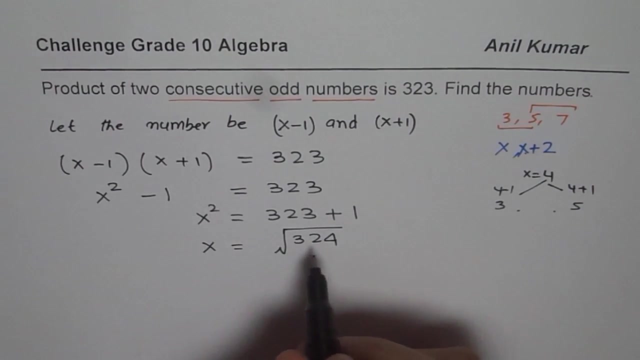 minus 1 equals to 323. now I can add one on both the sides, so I get x square equals to 323 plus 1, or I get x equals to square root of 324. right now, whenever you do square root, you should do plus and 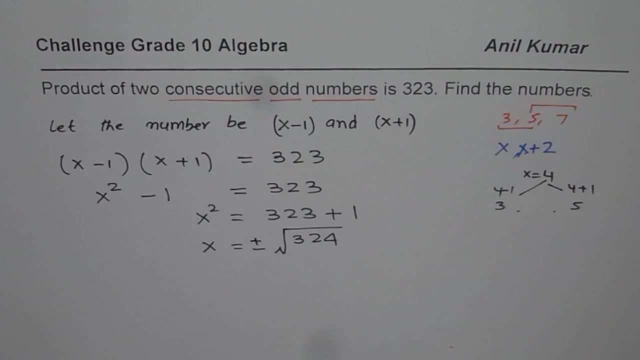 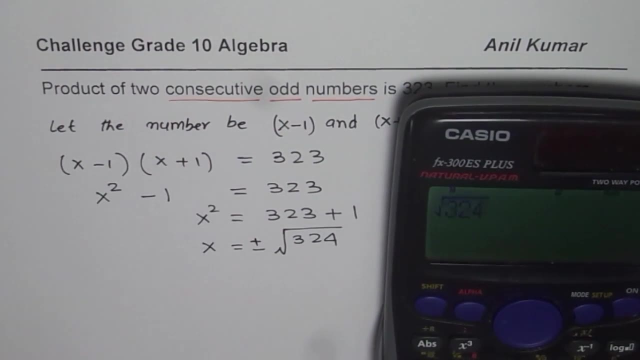 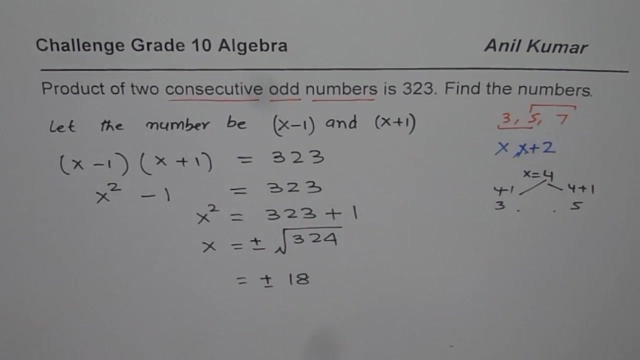 minus. okay, so when you do plus and minus, you expect two answers. for x, let us do square root of 324, so square root of 324 is equal to 18, so what we get here is plus and minus 18, correct, and therefore what should be the answer to this question is plus and minus 18, so we get x square. 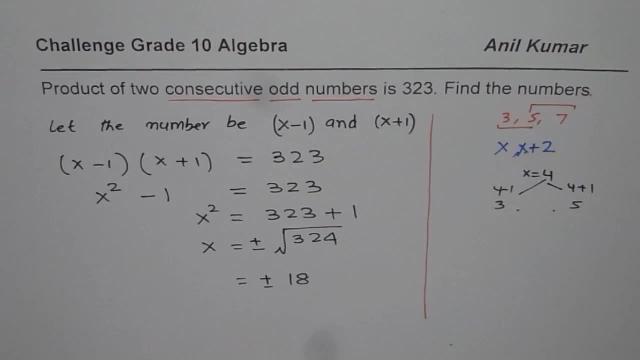 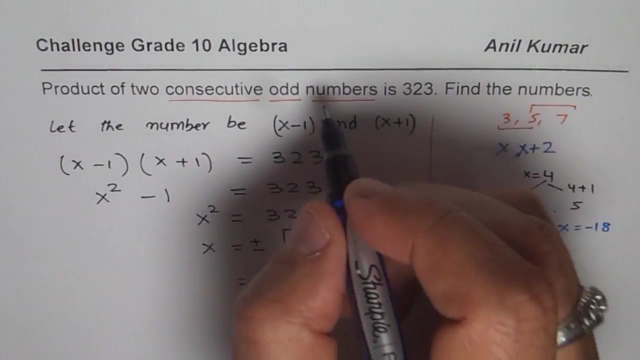 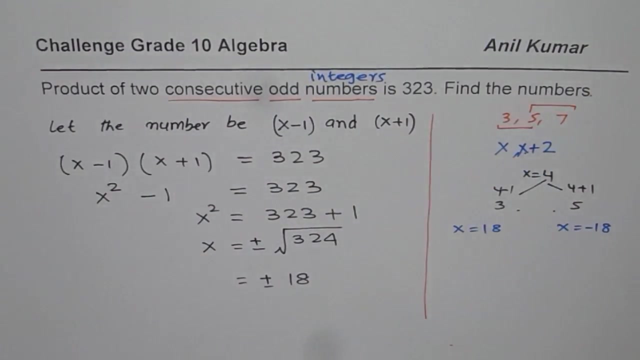 our numbers. well, if x is equals to 18 plus, let us say x equals to 18, we are taking plus, or x could be minus 18, right? we could have added here product of two consecutive odd. instead of numbers we could say integers also, right, that was a better term, so that it gives you a clear idea that we should also. 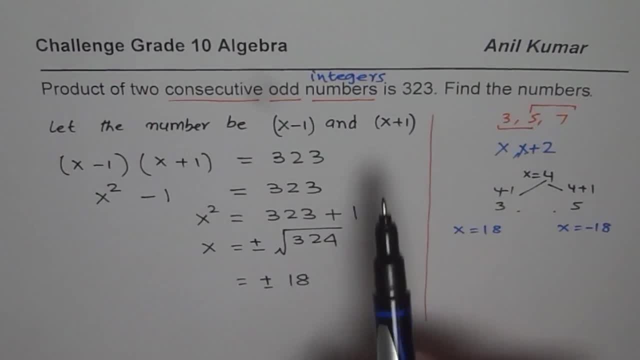 consider the negative numbers right, so I hope that is helpful. okay, so we have two possibilities: x could be plus 18 or x could be minus 18. if it is plus 18, then my numbers are: x: 1 equals to 18 minus 1, which is 17, and the other number is 18 plus 1, which is 19. 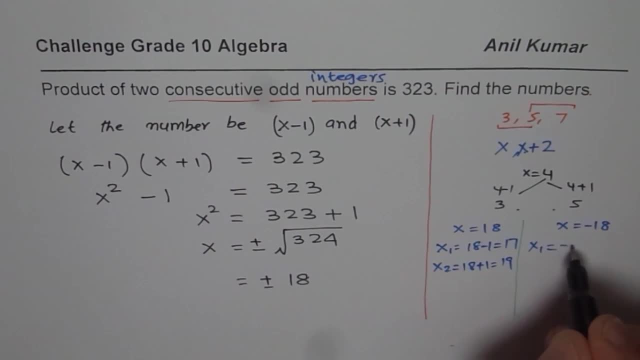 here the numbers will be x 1 will be minus 18, minus 1, which is minus 19, and x2 will be minus 18 plus 1, which will be minus 17. remember, if you multiply two negative numbers, you do get a positive number correct. so these are combinations of our answer.